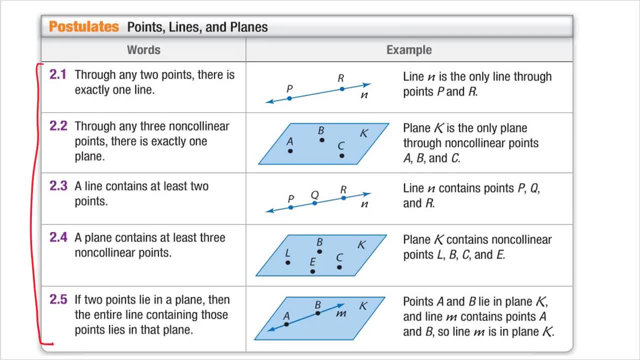 words for all the theorems- I'm sorry- for all our postulates, And then maybe draw the picture so that you understand what the concept is When we talk about these postulates. we're going to be writing these numbers, So you don't even have to worry about writing these numbers down. 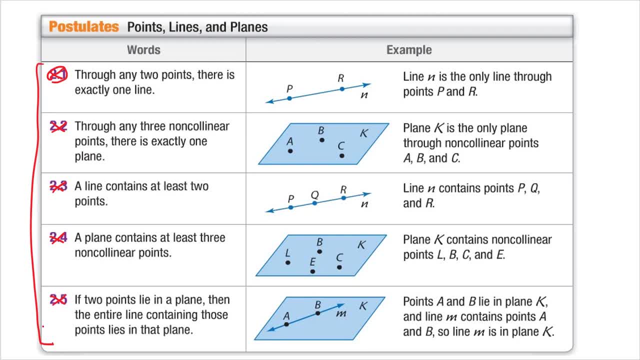 I never want you to say: be by theorem 2.5, because I don't know what theorem 2.5 is. I need to know what the concept behind that theorem is. Okay, 32 points. there's exactly one line. We've kind of talked about that already. So two points make up a line Through any three. 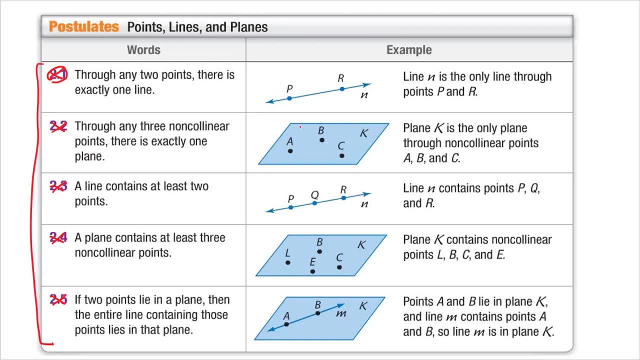 non-collinear points. there's one plane, Three non-collinear points. A line contains at least two points. Technically there is an infinite amount of points on a line. A plane contains at least three non-collinear points Again, 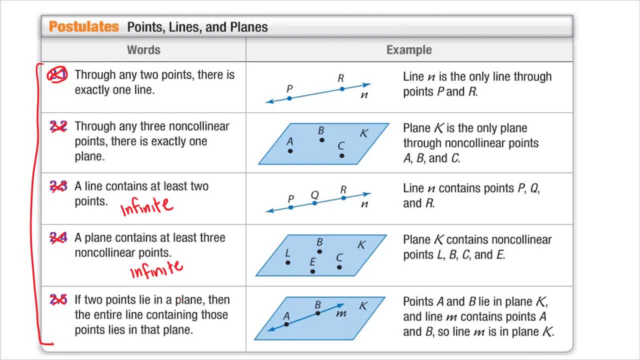 technically, there is an infinite amount of points on a line- I'm sorry, excuse me- on a plane. If two points lie in a plane, then the entire line is an infinite amount of points. So the entire line containing those points is on the plane, Okay, or is contained in the plane. 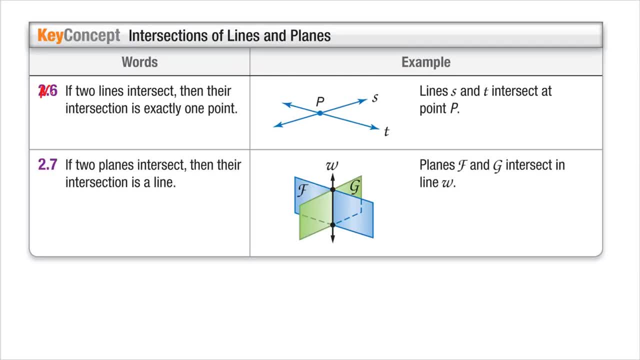 A couple more Again. you want to pause the video? write those down. We don't care about these numbers, but two lines intersect at a point, two planes intersect, their intersections align. Okay, understanding those concepts now- And I've kind of talked about those in previous. 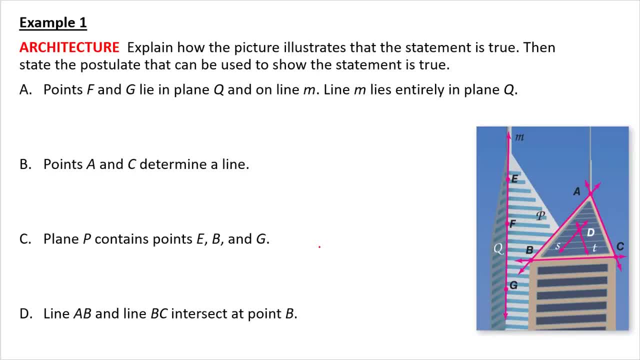 lessons. Let's look at an example here, Explain how the picture illustrates that the statement is true, then stated posture that can be used to show the statement. I look at this as like a picture of two buildings in a city. Points F and G lie in plane Q, so the side of this building here and on line F and G lie in plane Q. 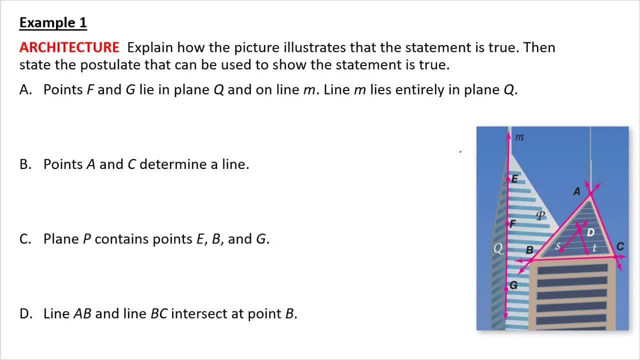 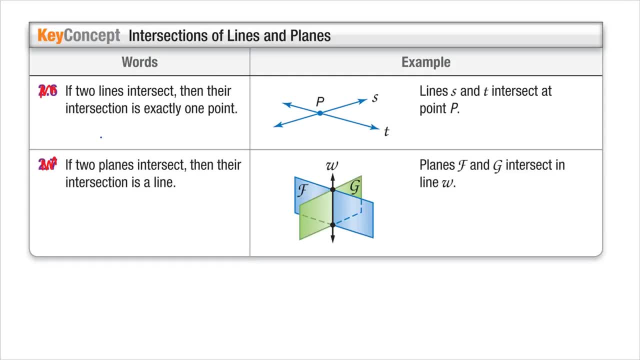 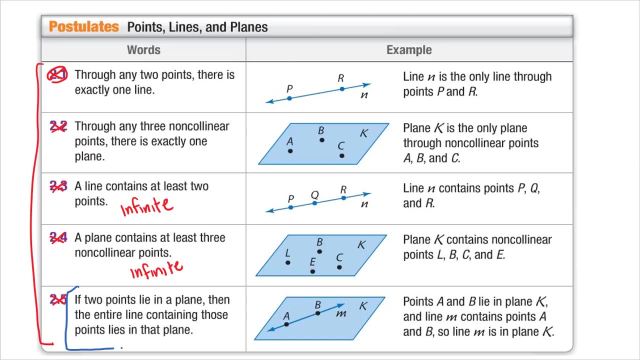 line M lies directly in plane Q. okay, so if that goes back to, you have to think of what theorem that goes back to. I'm gonna flip back to our theorems. it's talked about right here. two points lie in a plane, then the entire line. 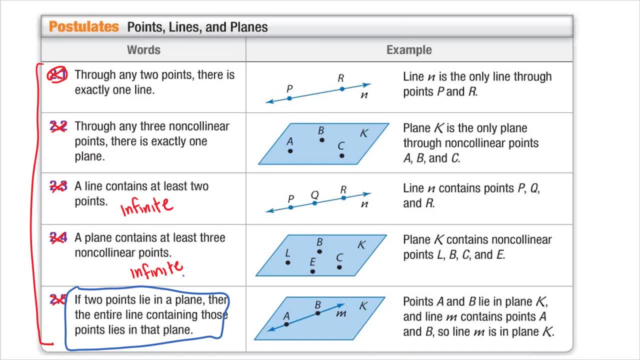 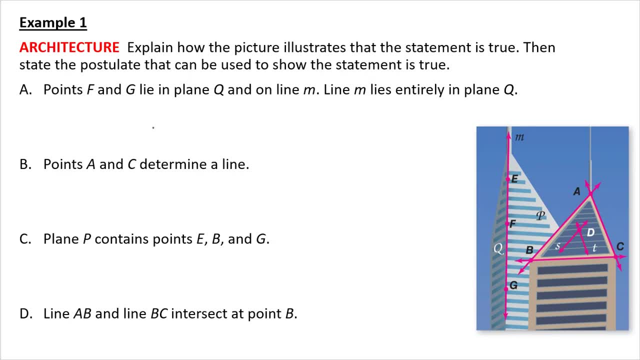 containing those pin, containing those points, lies in that plane. so now I need to write that. that's my justification here. so if two points lie in a plane, then the line that contains them is also in the plane. hey, these are like justifications. A and C determine a line. A and C determine a. 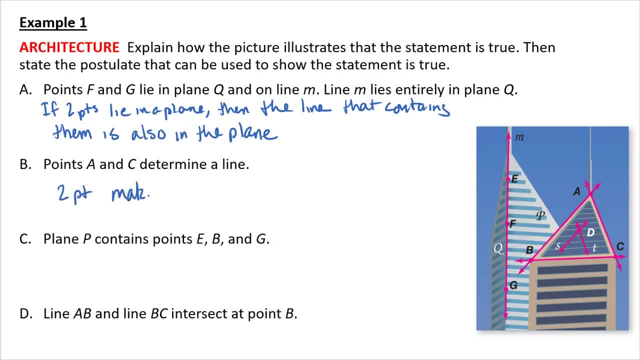 line. two points make a line. plane P contains points E, B and G. now I kind of disagree with this. I took this out of the book. but three non collinear. I think there's only one L in collinear. I think I was tired when I was. 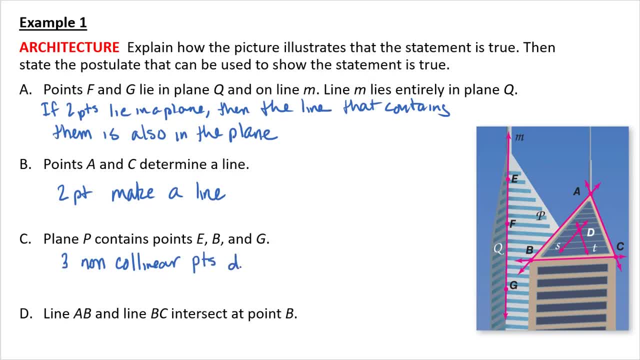 writing this. points determine a plane. if you look at this in terms of a building, It looks like points B is in a different plane in a different building as points E and G. But I can justify this: that E, B and G are all in the same plane because three non-collinear points determine a plane. 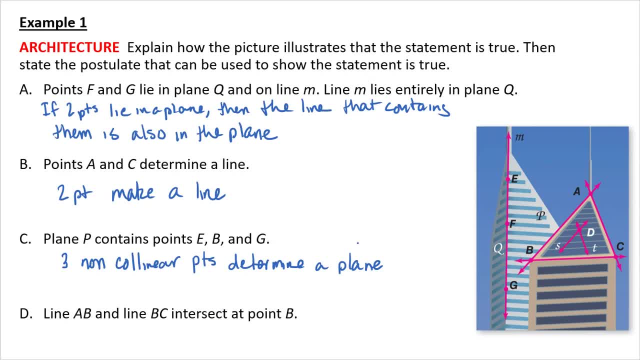 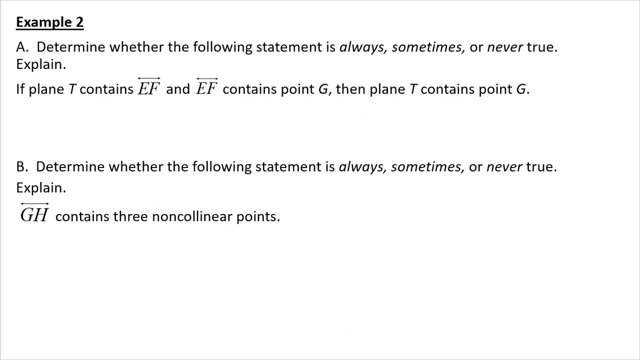 Okay, lines A, B and C and B C, A, B and B C intersect at point B. yes, because two points, two lines, I apologize. Okay. example two Determine whether the statements are the following: statements are always, sometimes or never true. 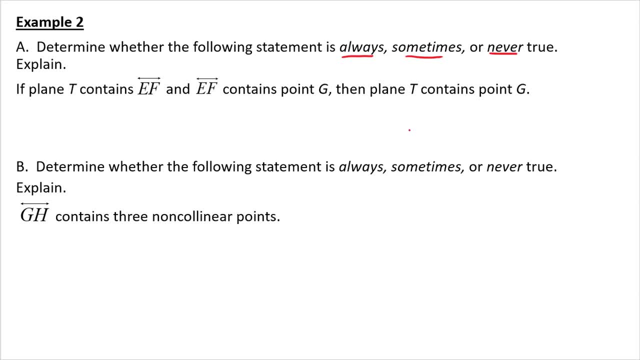 And I love these kind of statements- Plane T contains EF and EF contains point G, then plane T also contains point G. So I'm going to say this is always true And think about those theorems that we talked about. If a plane contains a line, then all points on the line are in the plane. 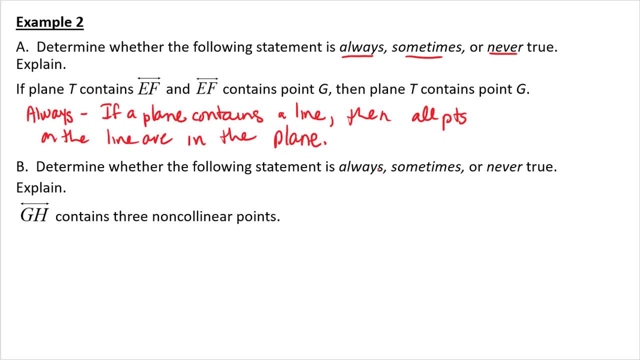 It's not a direct theorem, it's kind of like an offshoot of our theorem, but I'm okay with this explanation here And then determine whether the following statements- sometimes they're always never true. I guess I didn't have to have those directions again. 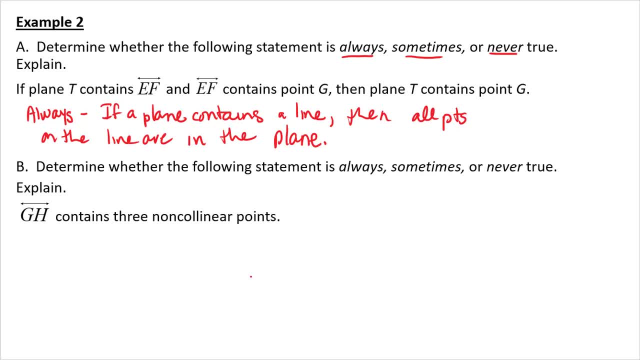 G, H contains three non-collinear points. Okay, That doesn't make any sense, because non-collinear points means not the same line, So this is never true. A that looks weird to me. Collinear points are are all on the same line. 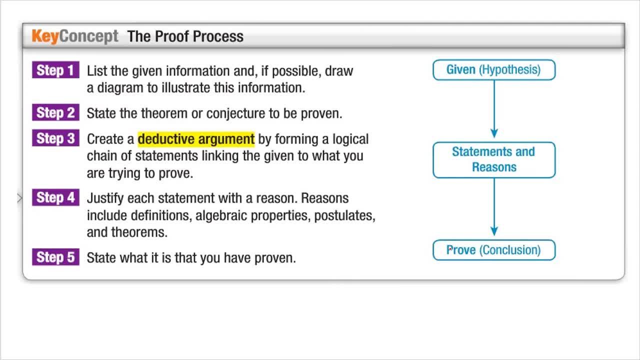 Okay, Proofs: We start off with paragraph proofs And then we move into two-column proofs. I prefer two-column proofs. I'm going to kind of glaze over a little bit on paragraph proofs for you guys. So the proof process, though, is really important. 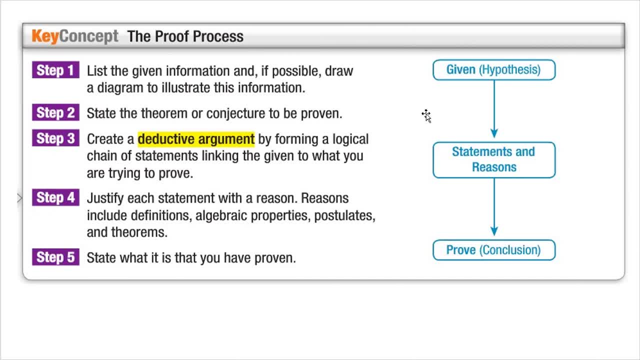 List the given information, if possible, and draw a diagram to illustrate. Okay, So the first thing you list is the given in any proof, And everything has to have. every proof has to have a diagram- State the theorem or condition. The argument is the only one that has to be proved. 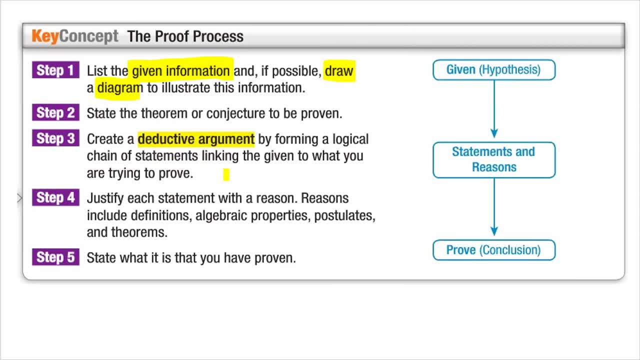 Create a deductive reason, a deductive argument. okay, from these proofs, definitions, Everything I've been giving you that will prove your statement. Justify each statement with a reason. Everything that you say has to have a valid reason. Our reasons, our definitions, algebraic properties, postulates, theorems. 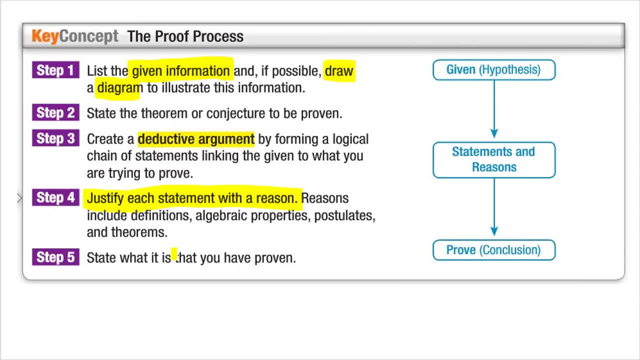 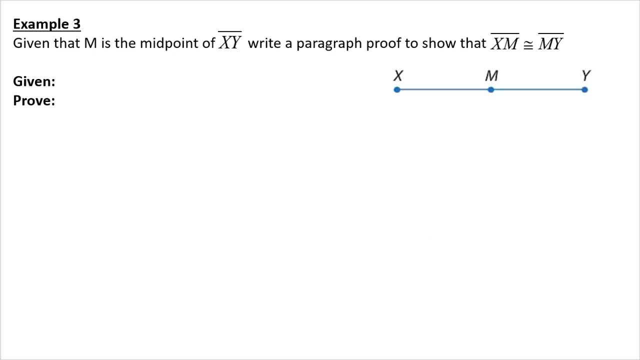 And then the last thing you say is the argument, The argument is the argument, The argument is the argument, The argument is the argument. last statement in your paragraph- proof is what you have proven. It says this is true because of this reason. 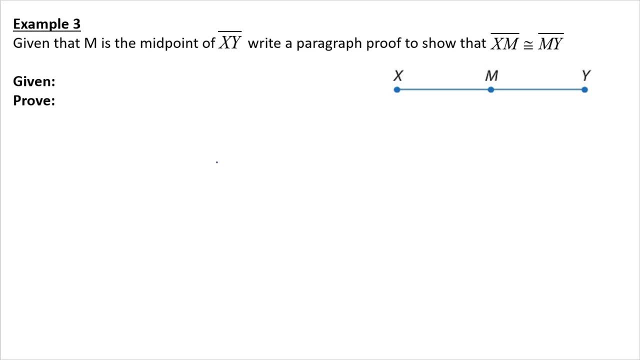 So let's do a paragraph proof. I'm not in love with this proof, but it's a good way for us to get thinking about paragraph proofs, Given that M is the midpoint of XY. given M is the midpoint of XY, So that's our given. 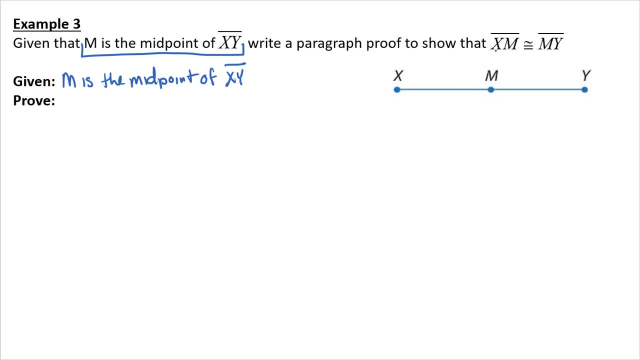 Write a paragraph to prove. okay, this is what I'm trying to prove, Okay. So, And notice how I have a given, a proof, and I have a picture over here. A lot of times I'm going to be braiding out these given and the proofs for you and I'll 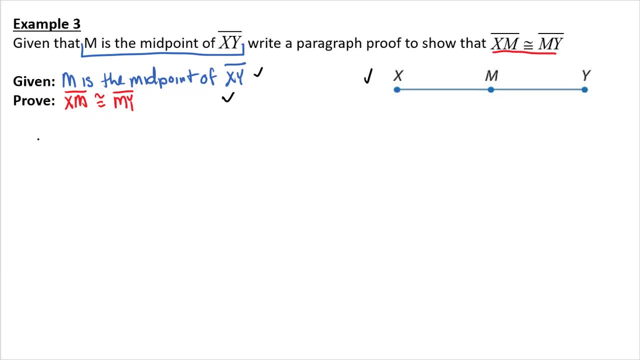 have the picture drawn. Okay, So our proof: a midpoint Splits a segment into two equal parts by the definition of midpoint. Ooh, I don't like what I wrote there. What I'm going to do, I'm going to take this. 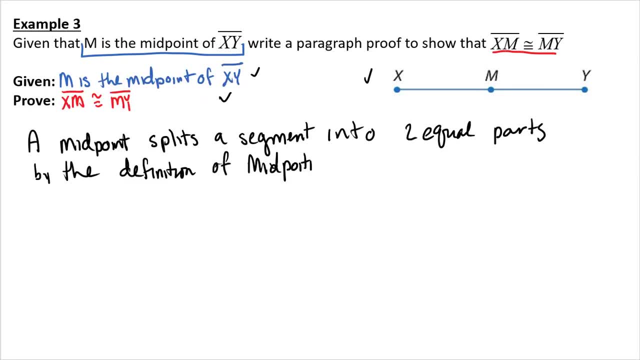 I can't move it down. I was going to try and move it down By the definition of a midpoint. What I don't like that I just wrote is I first have to start with the given, So my first sentence should be: we are given that M is the midpoint. 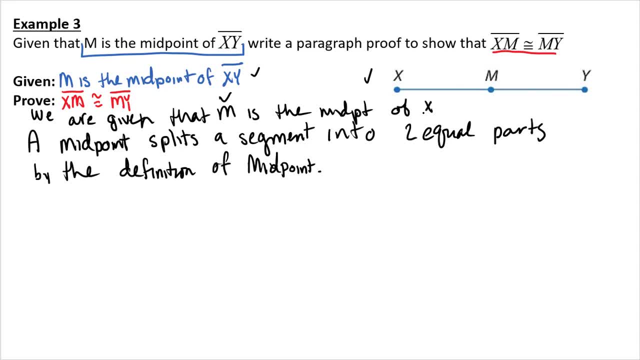 Okay, Okay, So that would be M of XY. Okay, So first just write out your given, then you say something about that. A midpoint splits the segment into two equal parts. by my reason, This is my reason right here. So then we can say therefore: 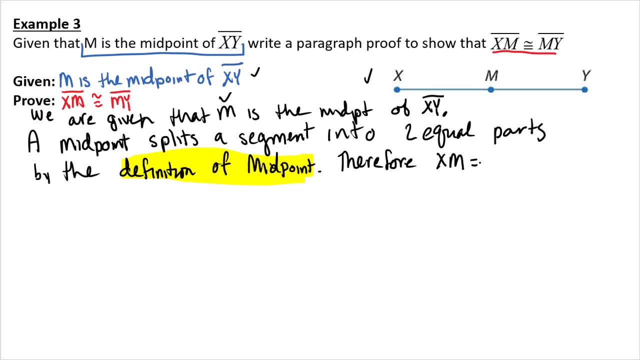 XM equals MY. Okay, All right, I got it Okay. Okay, I have two equal parts. By the definition of congruence, we have xm is congruent to my. Okay. why I like this proof? Because I like it. because you have to start out by saying you're given, saying it splits. 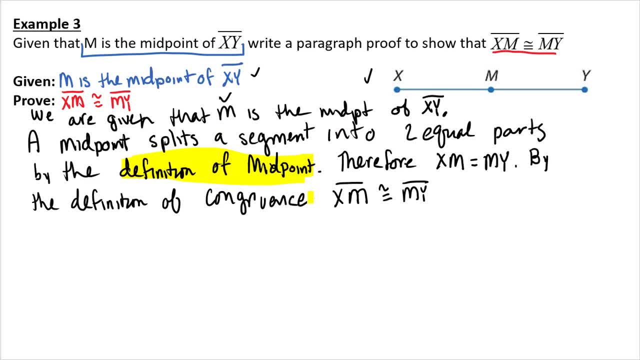 into two equal parts, Something that I am not as picky on as other geometry teachers. okay, Other geometry teachers are different than me, and that's okay. They can be picky on this, And our book does this, but I'm not going to be as picky, okay. 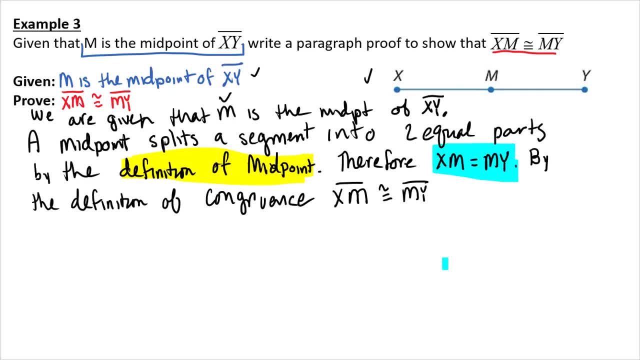 If you have this segment- lengths are equal- and you're trying to prove congruence, You have to then state they're congruent by the definition of congruence. okay, And our book is just kind of a stickler on that and some geometry teachers are sticklers. 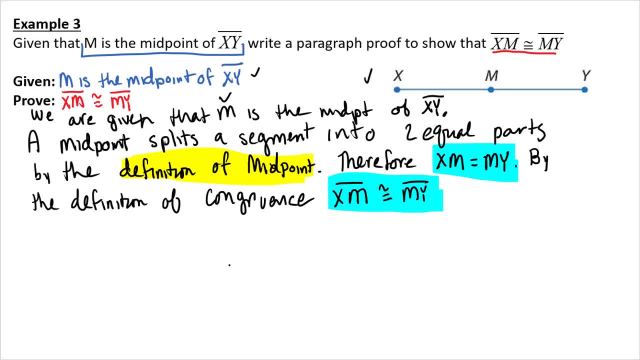 on that. I am not as big of a stickler on that, okay, That's why this is maybe a little bit weaker of a proof. But now that I know that we've proven a theorem, now We've proven that if m is the midpoint, then I have equal congruent segments. I should 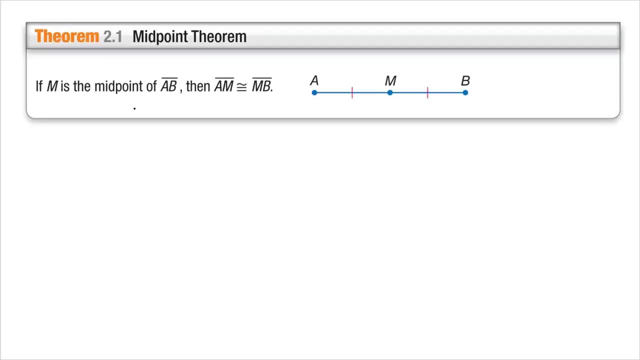 say So, We have our midpoint theorem. okay, This was our hypothesis. The if part was our hypothesis. We proved this. We proved our conclusion And make sure you have that midpoint theorem written down in your notes. We're going to be using that a lot as we move through the different proofs that we're going. 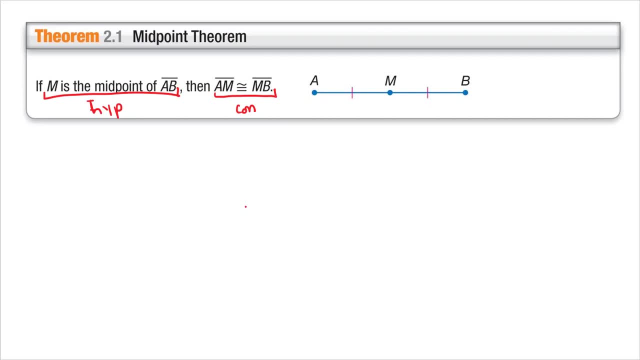 to be doing. Okay, So that is our postulates And paragraph proofs lesson. Thank you for watching.